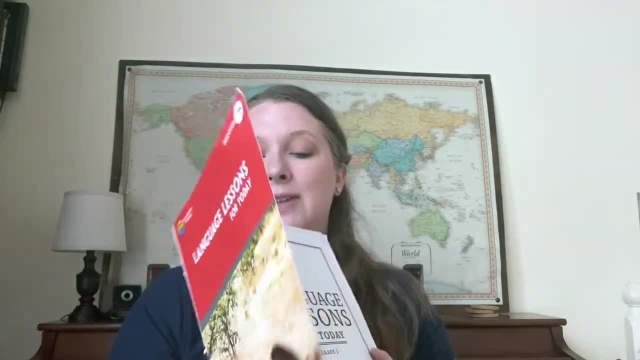 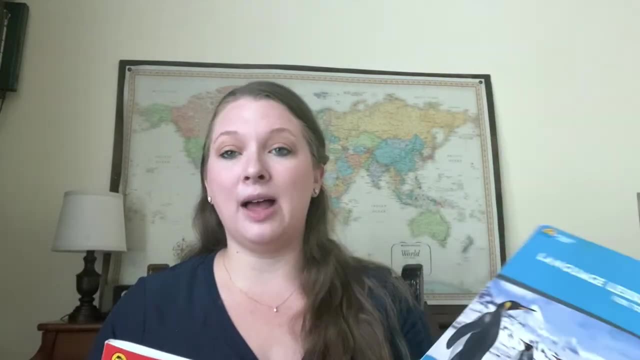 rough on things, so the binding came off of his book and I need to to reattach it, but my fourth graders is still holding up really well. my sixth graders is actually spiral bound and it's holding up pretty well too. I can pass these down. 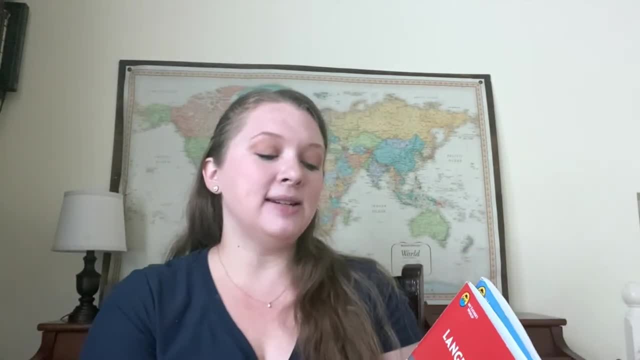 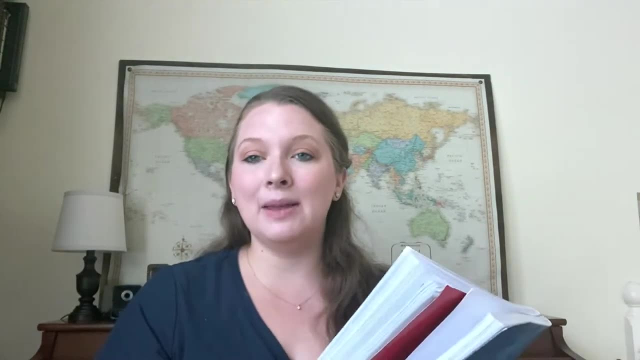 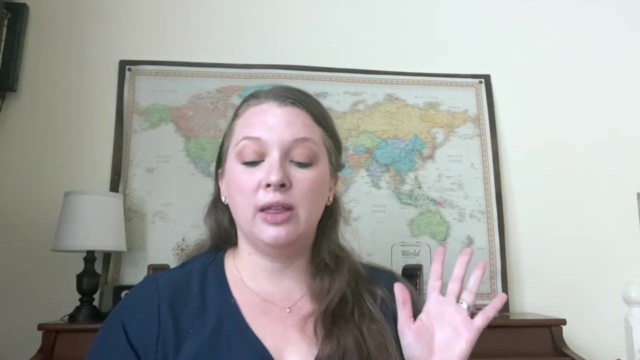 to my kids, my younger kids, and, yeah, not have to rebuy the program every single year. now, how I did it was anytime that my kids needed to write anything down. they had a spiral notebook that was set up just for their language lessons, for today stuff, so they would write the lesson at the top of the page with the 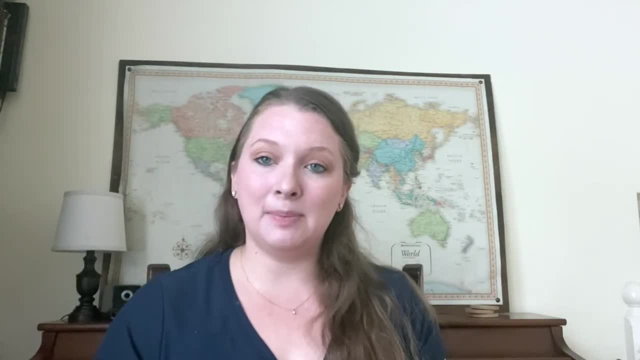 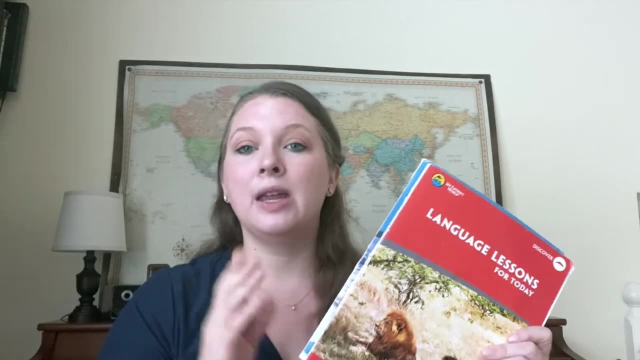 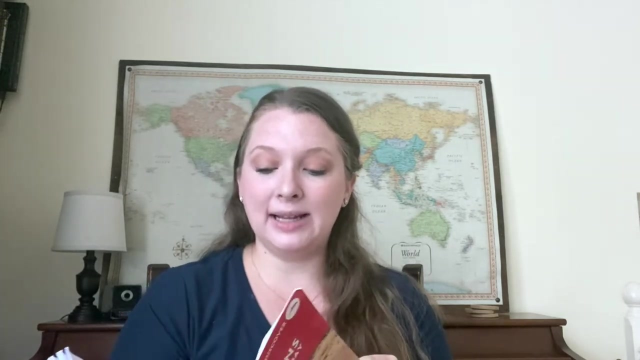 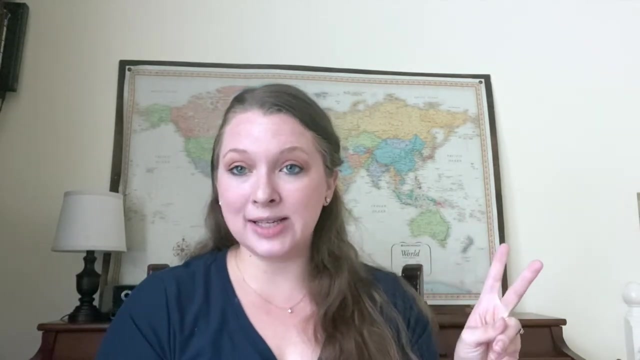 dates and then complete whatever it is that they needed to complete. now they don't have to write for every single lesson. this is not a writing curriculum: language lessons for today. grammar: it does cover some composition, but they're not going to actually, you know, be writing essays with this. they do copy work poem, memorization picture. 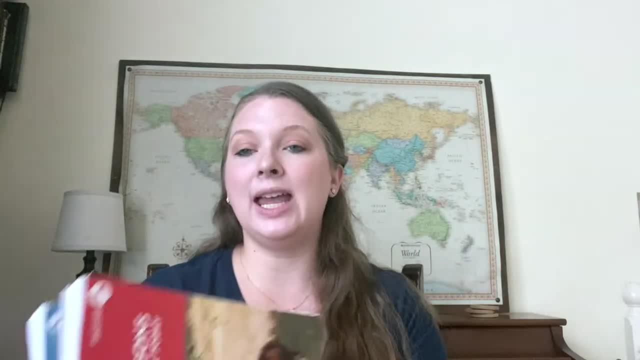 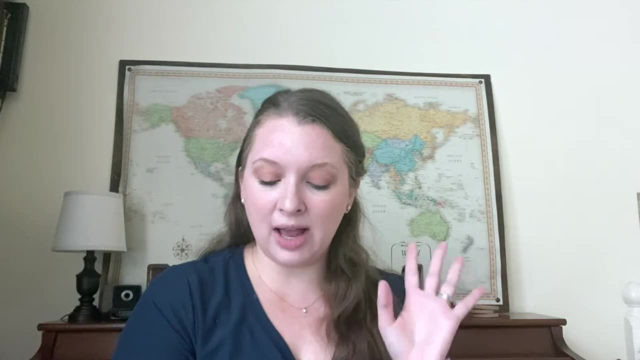 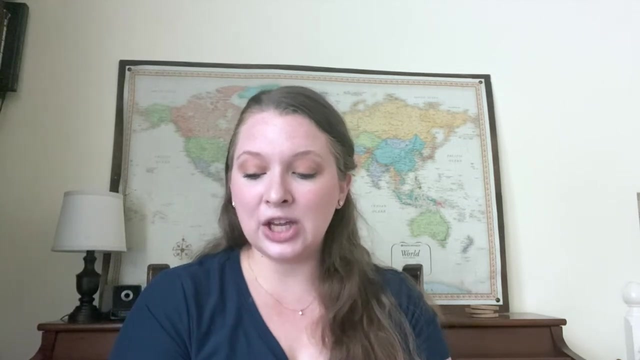 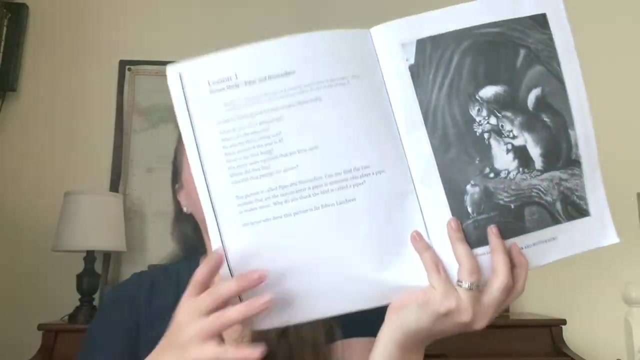 study a lot of oral composition, especially in the younger years. letter writing, they work on abbreviations, all kinds of grammar work and all of that stuff, and it is covered in a short, easy to use lessons. so, for example, here is lesson one in grade two and this is just 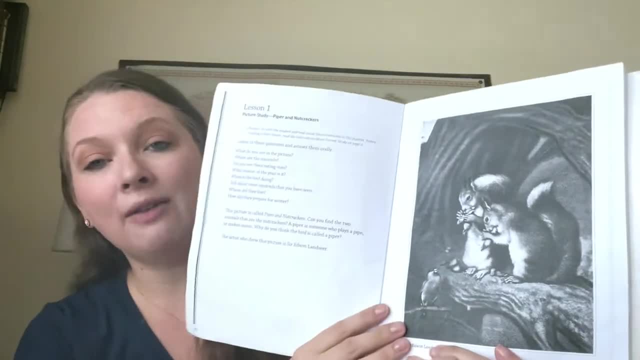 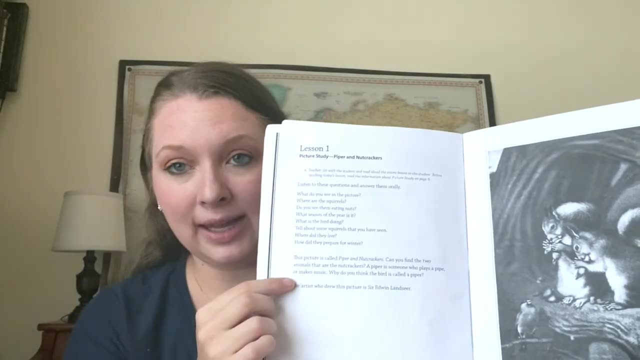 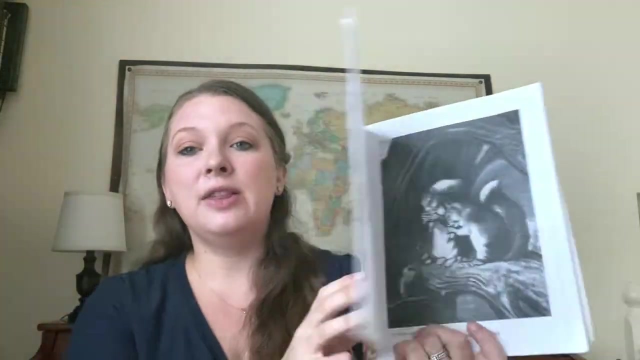 a picture study, so, and they do have color pictures as well. so your child will study the picture and then they will answer these questions orally. keep in mind this is for a second grader, so there's not a ton of written work in grade two. this approach is very similar to the one that I showed you in grade two. 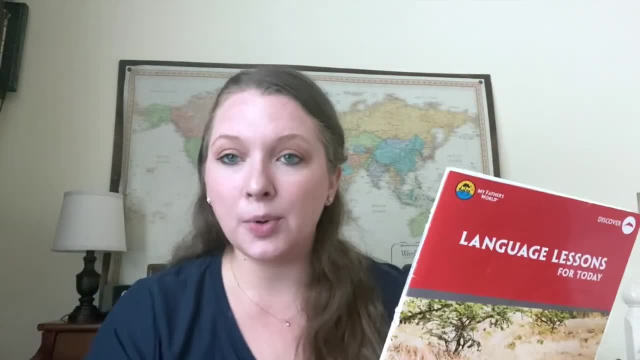 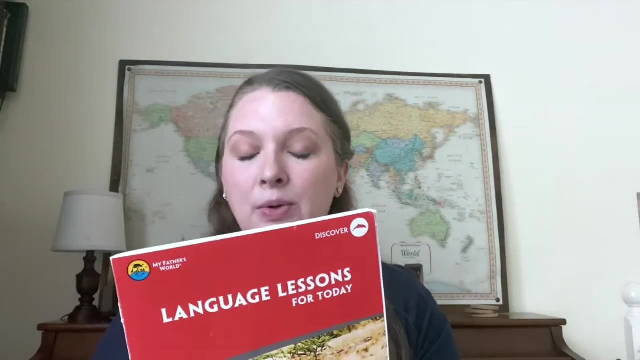 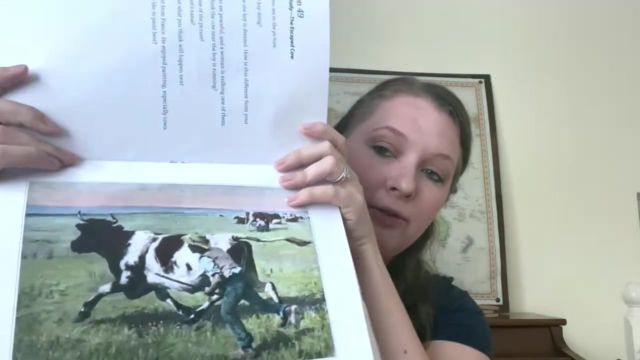 this approach is very similar to the one that I showed you in grade two. this is similar to a Charlotte Mason approach to grammar and English, basically, as well as some classical approaches. so there's dictation included. here's a color picture for picture study, and every day they're doing something different. so one 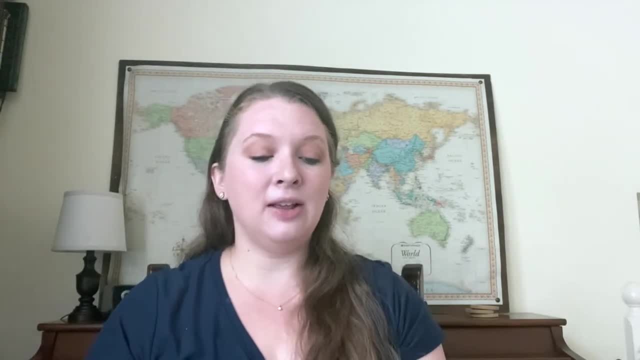 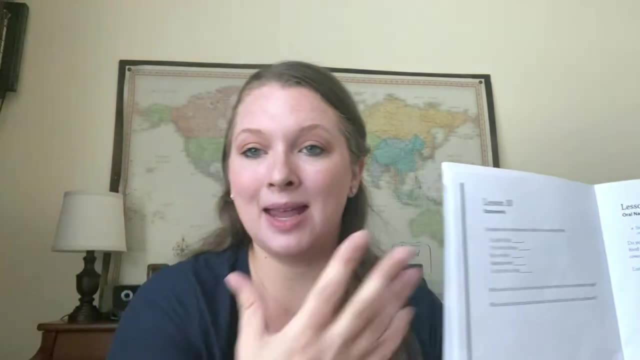 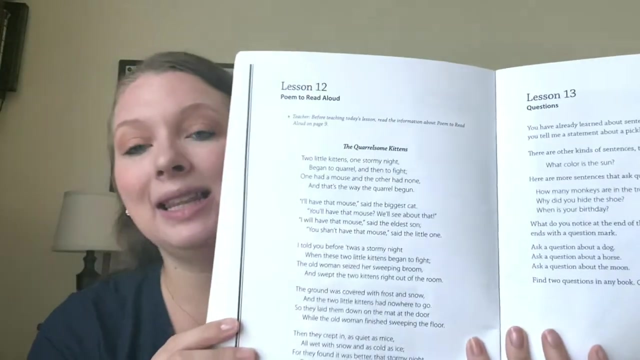 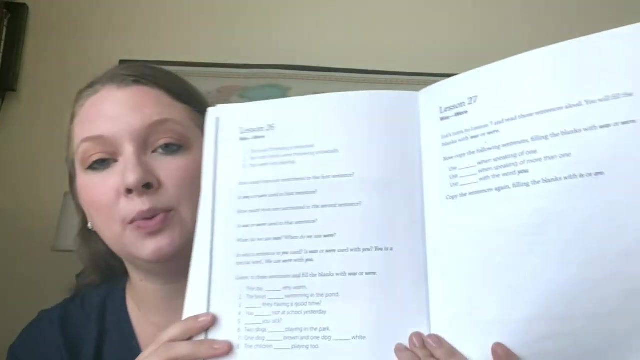 day they'll be studying a picture. the next day they'll be working on statements and filling in the blank and learning the difference between a statement and a question and an exclamation. there's poems to read aloud, different poems in here for them to memorize, and the difference between was and were the. 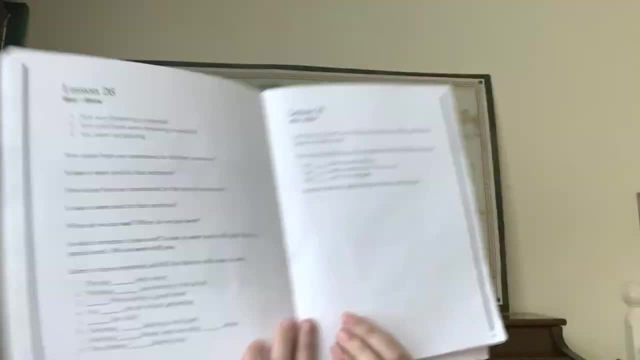 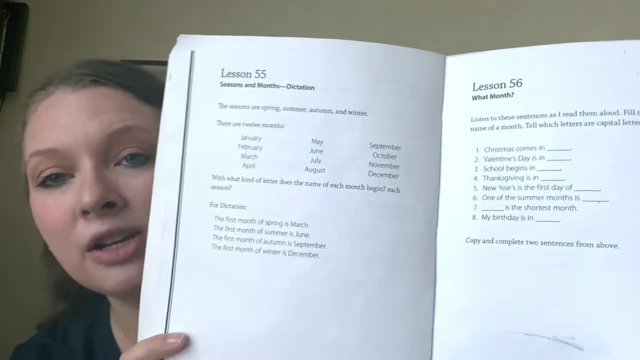 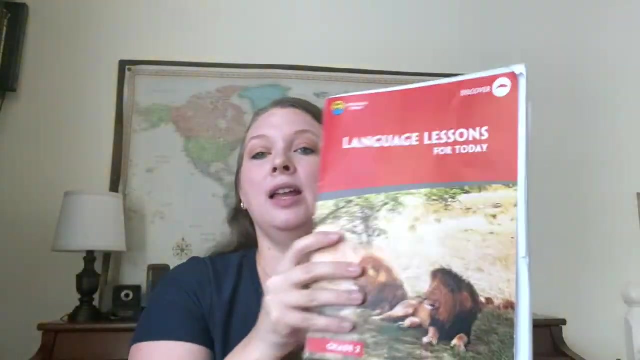 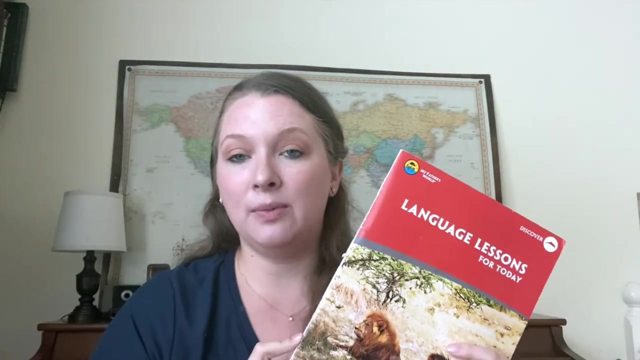 difference between a and and the articles. they'll learn about different articles, different pronouns. here's a look at some dictation further on in an. This is Seasons and Months Dictation and overall, like we spend maybe 20 minutes a day doing our language lessons. Now my second grader does not do a separate writing curriculum. 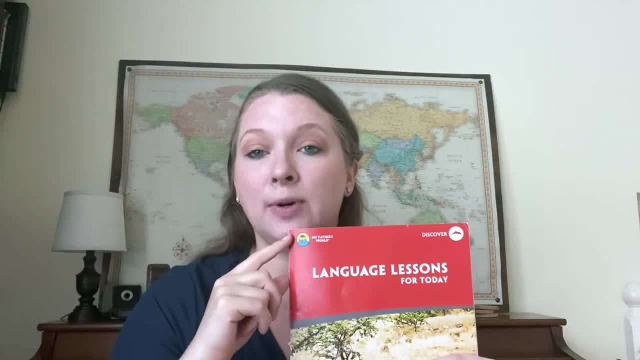 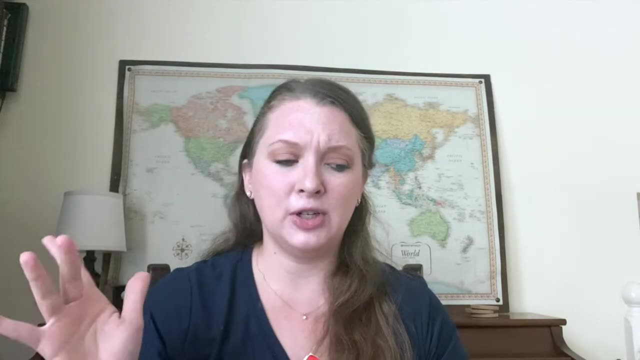 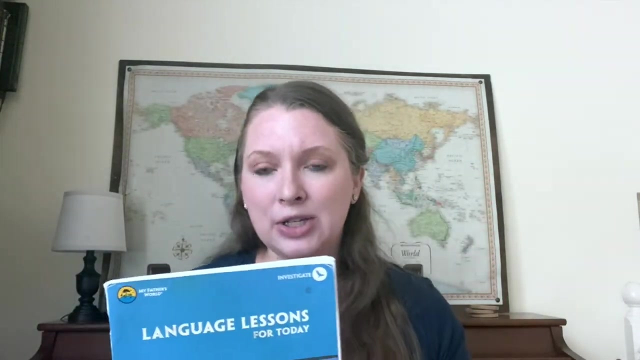 My fourth grader and my sixth grader do language lessons for today three days a week, and then two days a week they will use my father's world's writing skills. for today is what I think it is, and it's kind of a companion which I will. if you guys want me to, I can do a flip through and 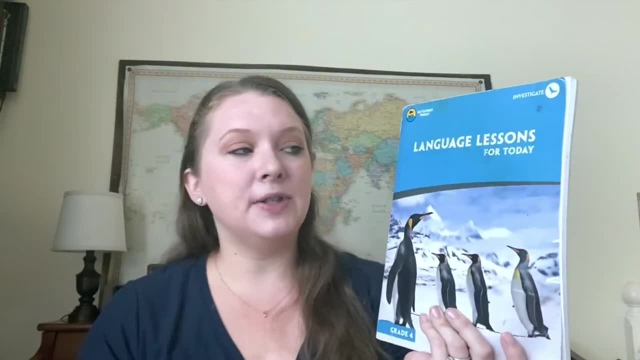 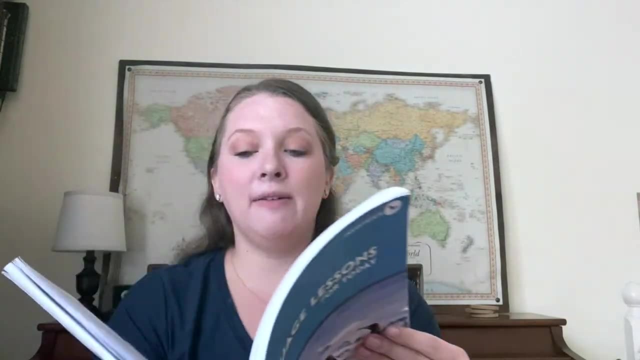 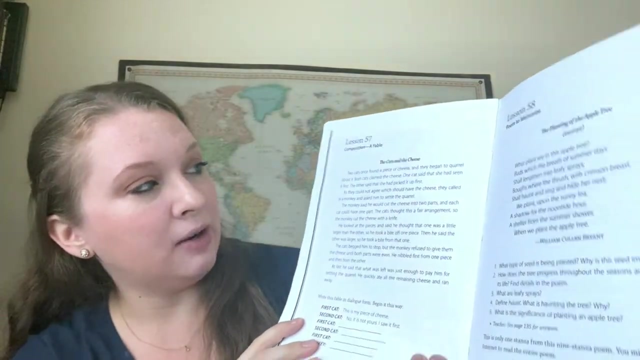 a review of writing skills for today as well. So that's just for the older children in fourth grade and above. Now here's the fourth grade book and it's set up in a very similar way but just a little bit more complicated than the second grade book. So here is a composition, a fable. 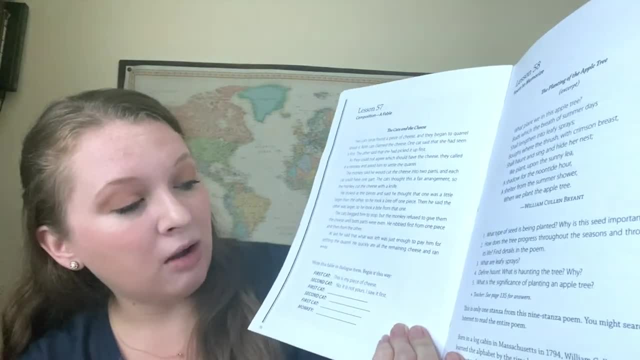 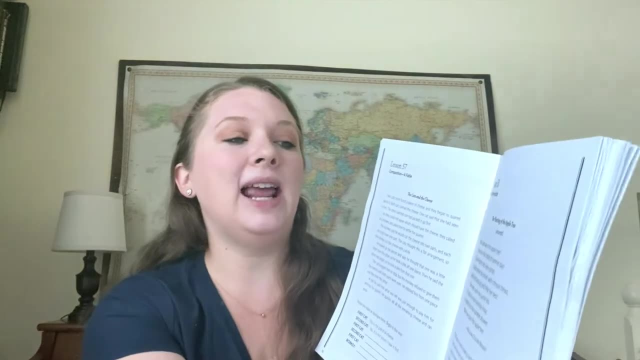 and then it says: write this fable in dialogue form. begin it this way. So they in fourth grade. they're beginning to learn dialogue and quotations and how all of that works. Here's an example of a poem to memorize: 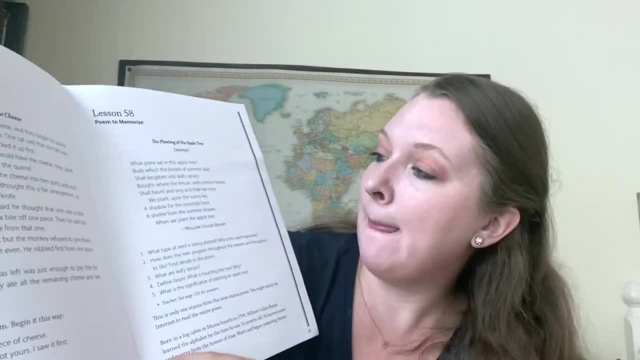 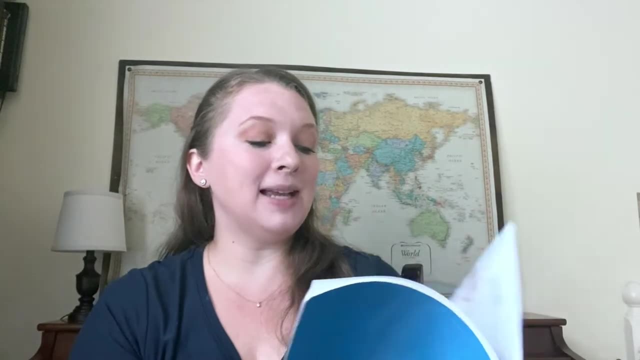 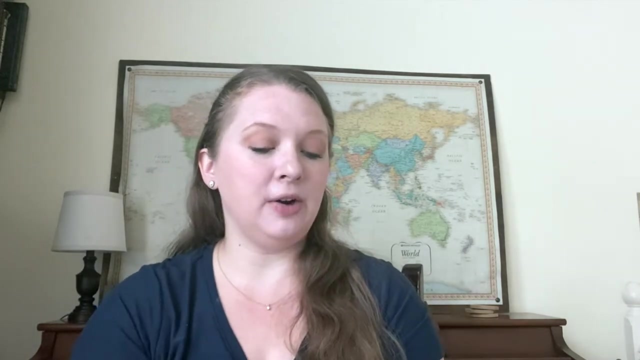 So we have the planting of the apple tree and there's an excerpt, some questions being asked My sixth grader. so I did notice with my fourth grader. they didn't keep a separate envelope, a grammar envelope, I'm not sure what. 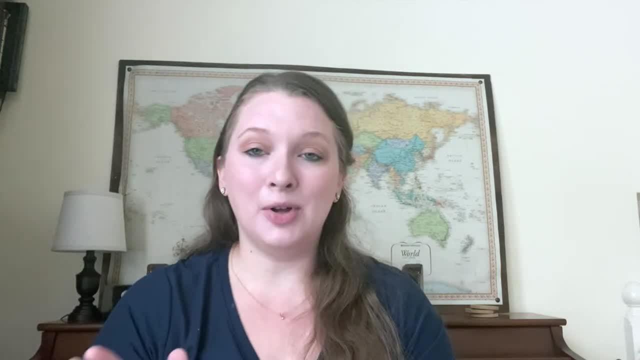 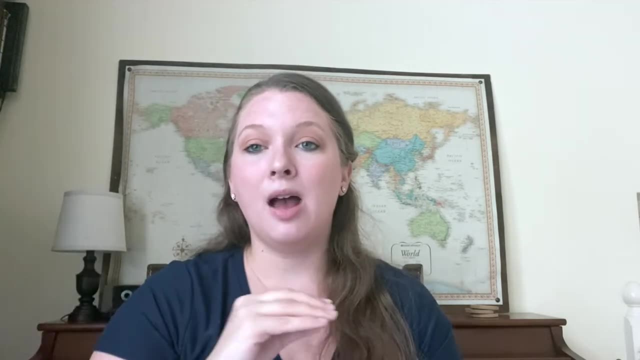 happens in fifth grade. yet I haven't looked at the fifth grade book, although we do have it, but my sixth grader did keep his own grammar envelope. So he would write down a particular part of speech, whether it was an article or an adjective or whatever. he would write that on the 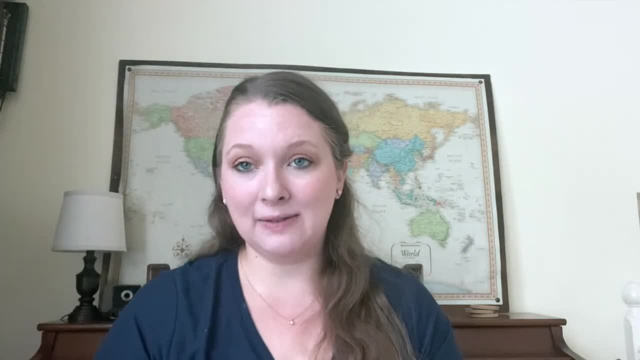 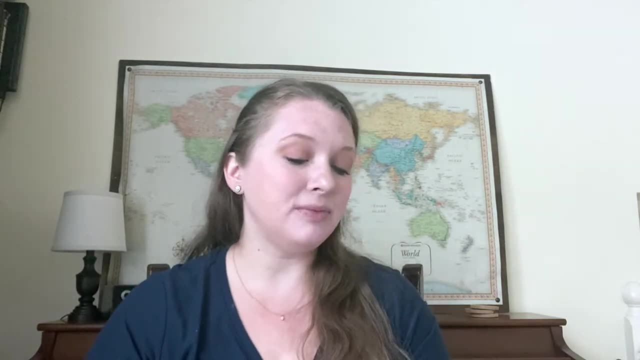 front and then on the back he would write the definition as well as give some examples, and he would keep those in his envelope and then he could go back and refer to them if he needed to. So that was one way that he was learning his grammar. Here is an example of a poem to read: 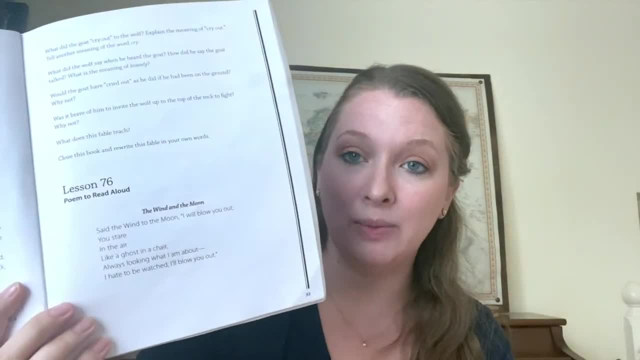 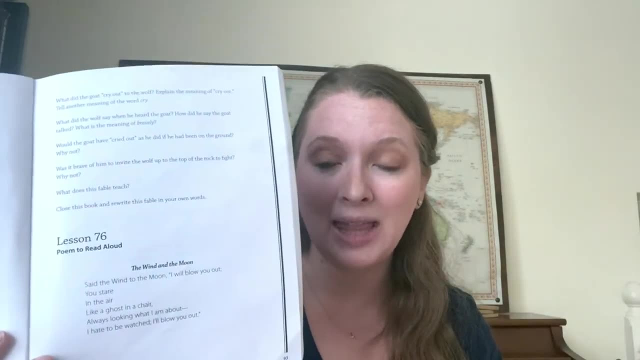 aloud. Now I would have her. since she is reading very well, I would have her read this poem aloud. My second grader is reading very well too, so I would have him read his poem aloud. If I had a child that was still not a confident reader, I would read the poem aloud to them. 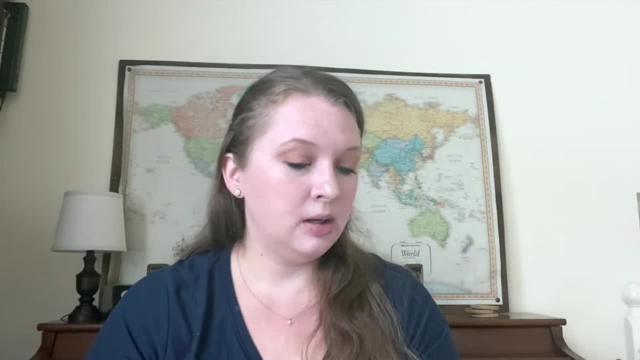 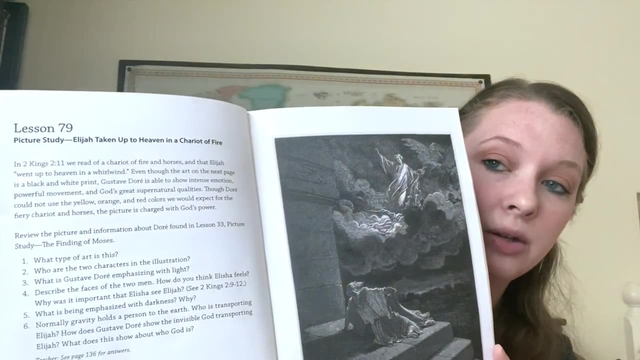 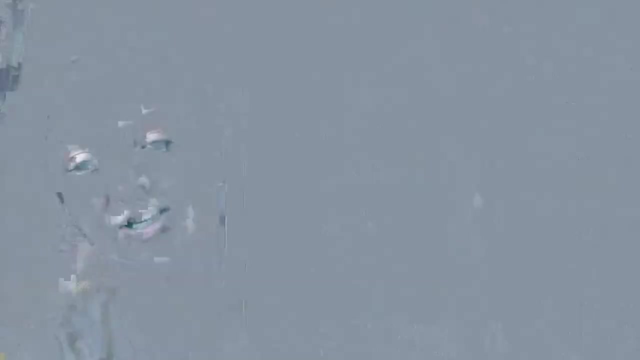 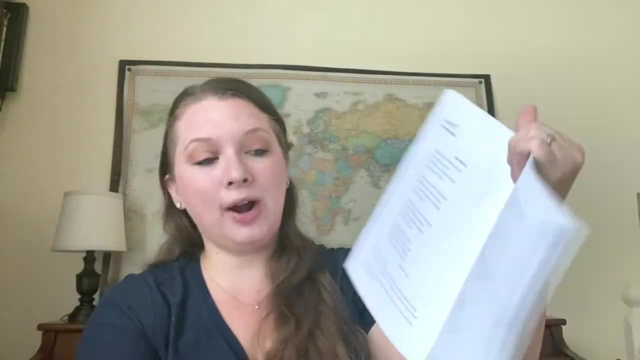 Um, let's see. Here's a picture study example in the fourth grade book and a poem to memorize. So, as you can see, it gets a little bit more complicated. This is a longer poem than one that would be found in the second grade book. Also, we worked on a lot of different books. It is decide upon things, but we really looked at them. Let's see. Let's open it up here. All right, I'm going to add something to this. Brian Nugent, and reading what was set in the fourth: grade book, Nathan Eddison. So these are the first twobooks. This book is named Christiano and I am also a three-year grader and I read these three books, a first and a third slash. I want to just say that it is great to book. 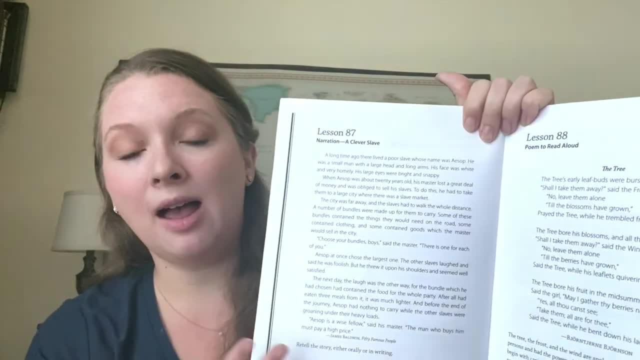 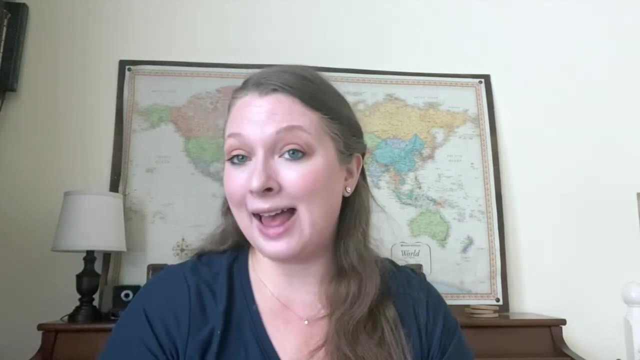 Okay, This is a good introduction between three chapters narration. so the child would read a composition and then narrate it back to me. a lot of this was done orally. they had the option of doing it orally or in writing and you know, whenever they had to write, like I said, they would just 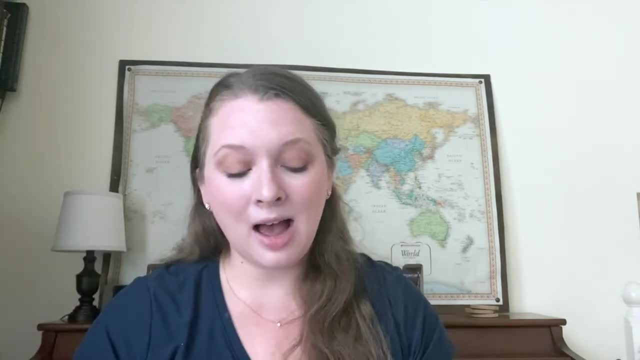 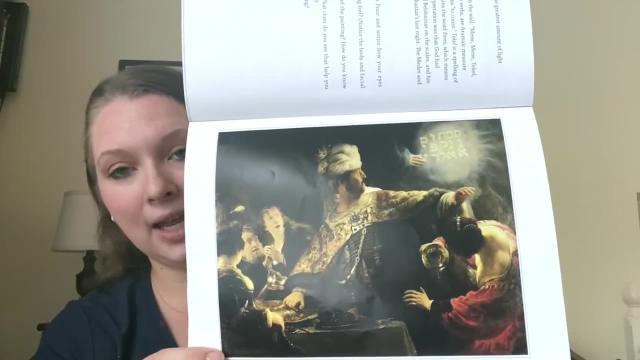 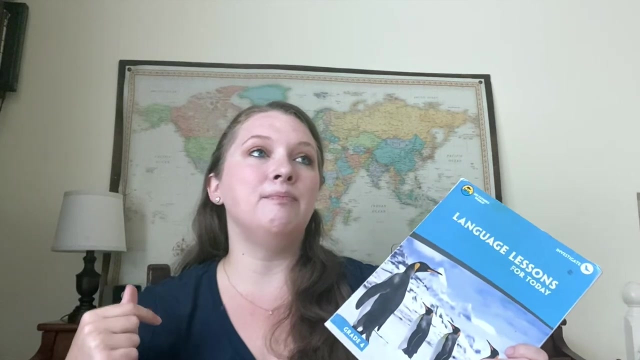 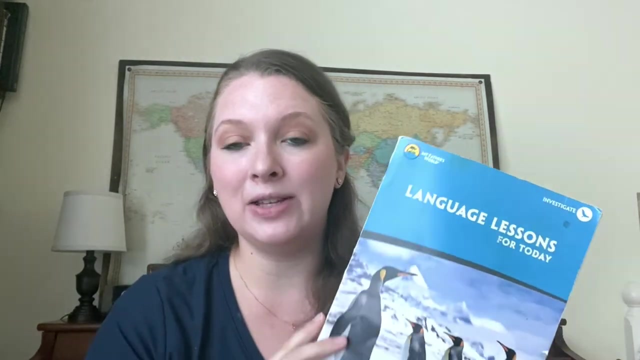 pull out their spiral notebooks, write the lesson at the top and then fill in whatever it is that they needed to fill in. here's a another example of a picture study. so this covers all of that great stuff: picture study, poetry, grammar, narration, dictation. that's why I love it so much and it doesn't take long at all. 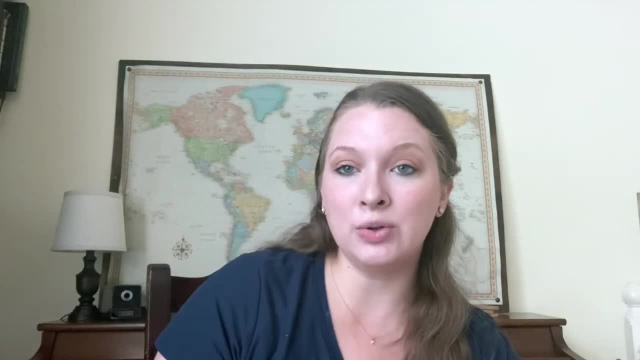 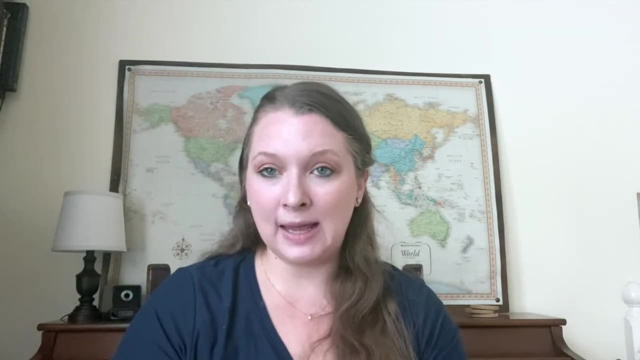 to complete the lessons and it really flows for our homeschool day, in particular because I have so many students that I'm trying to teach now. it doesn't cover geography, it doesn't cover spelling and it doesn't cover grammar and it doesn't cover grammar and it doesn't cover